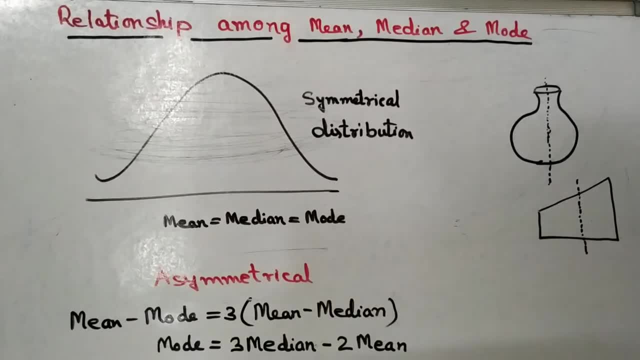 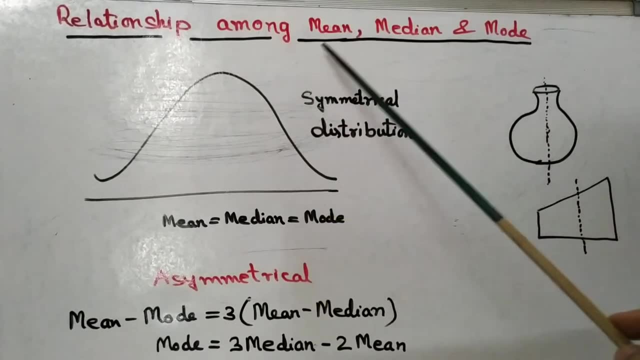 Hello students, today's topic is relationship among mean, median and mode. That means the relationship among the three central measure of central tendency, that is, mean, median and mode. So before knowing the relationship among these three measure of central tendency, let us know what is symmetrical or asymmetrical figure. I have drawn here two figure. First, 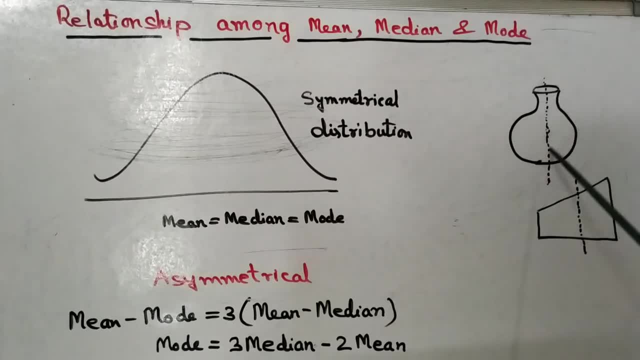 one is symmetrical figure because when we cut it from the middle, we get the same shape on both the side. Now here in the second figure, this figure is asymmetrical because when we cut it from the middle, we get different shape on both the side of this line, This figure. 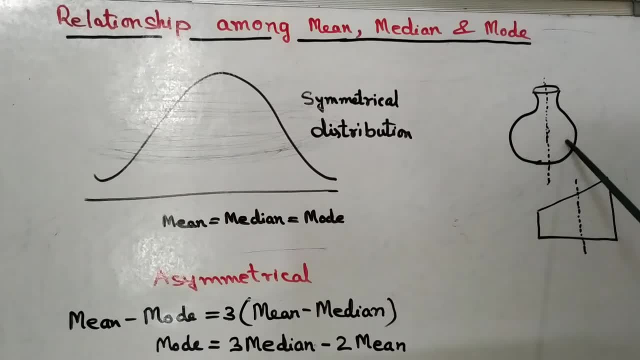 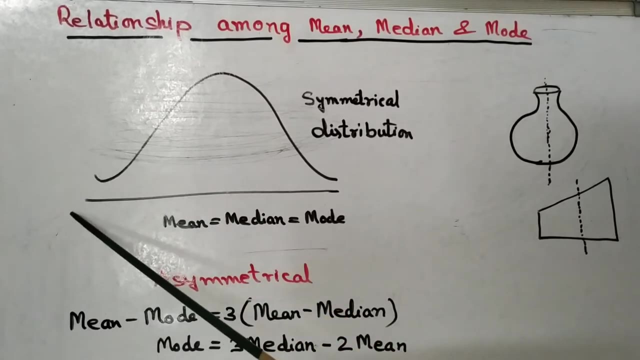 is different, this figure is different, but here the figures are same, The shape is same. So it is a symmetrical figure and this is a asymmetrical. Now, when we plot the graph, when we plot in xy plane, if we take x along x axis, that 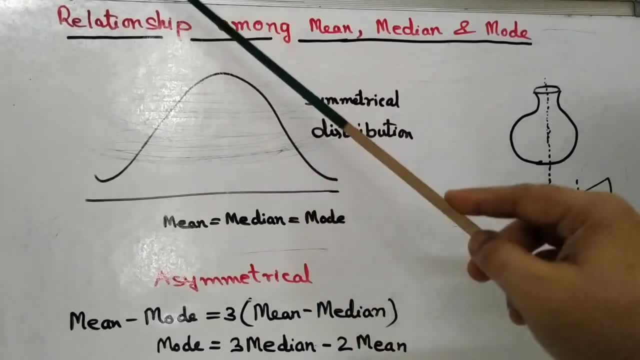 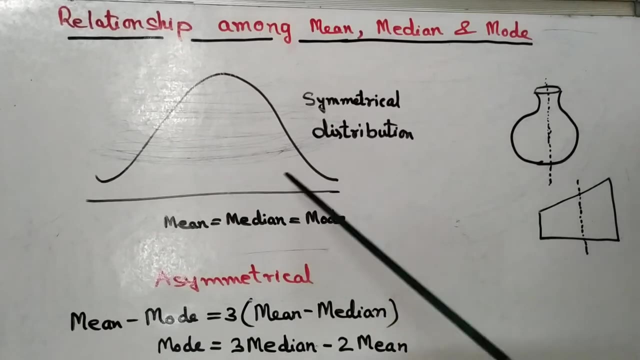 means the variable along x axis and the frequency along y axis, and if the curve is like this, then it is called symmetrical distribution. That means when we cut it from the middle we get same shape on both the side, So it is a symmetrical figure. 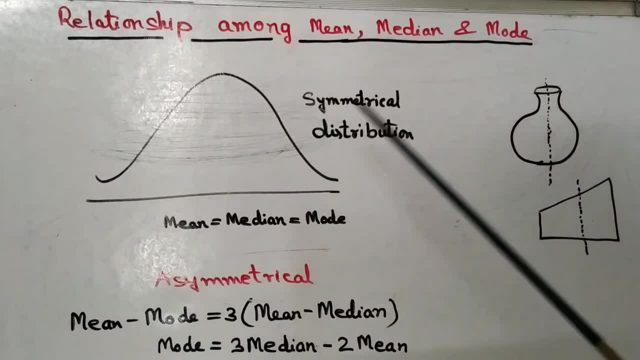 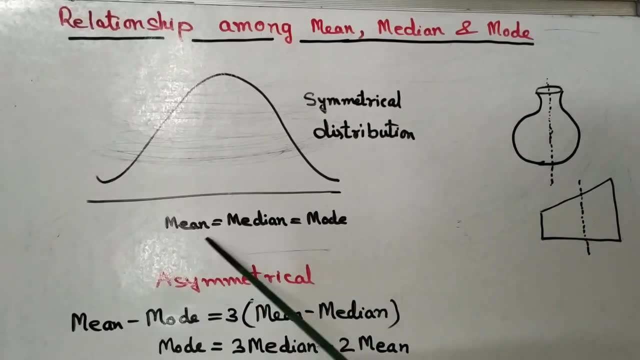 So wherever we get the shape like this, it is a. it is called symmetrical distribution, And in that case mean is equal to median, is equal to mode. That means all the values are equal. That means it comes at one place. Okay, Here, the highest frequency is here. 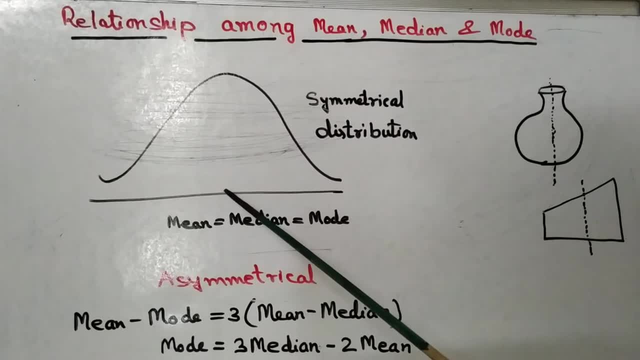 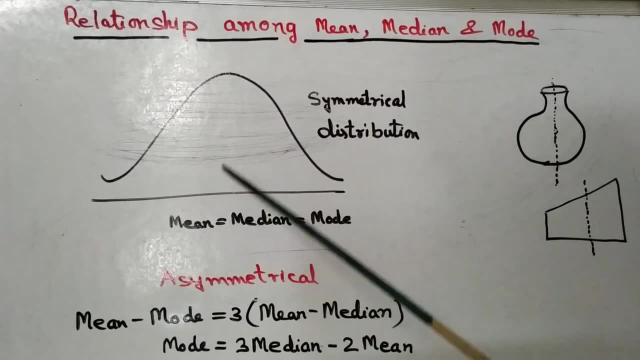 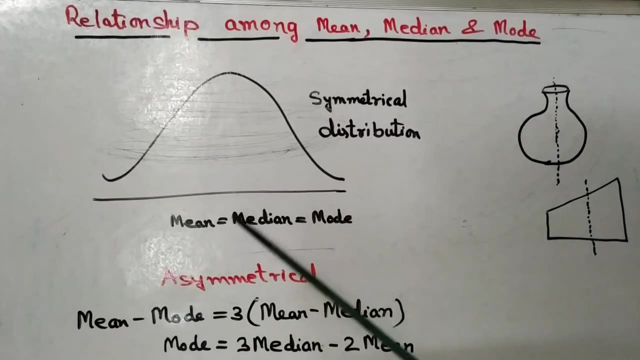 So mode will be here. That means mode value will lie here. So all the values- mode, medium, median- divide the observation into two equal parts. So we get median also in the central, Okay, And mean also. So the values are here at the same, it lie at same place. So when, whenever we get a 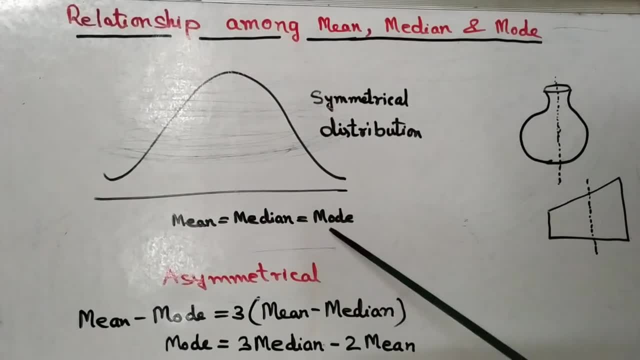 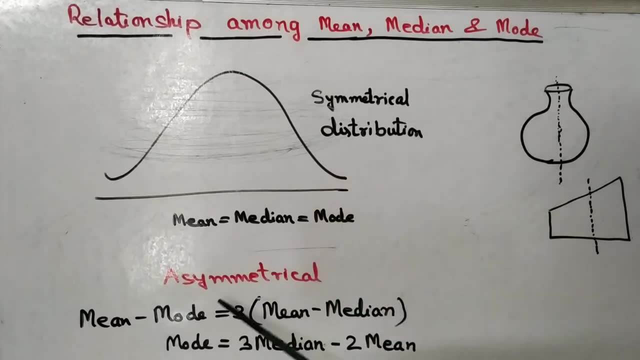 symmetrical distribution. we get mean median. the relationship among mean median and mode is equal. All are equal. So now a symmetrical figure. Okay, Symmetrical means when the figure is of different shape. That means if it is slightly skewed, this positively side, or this is skewed negatively side, or